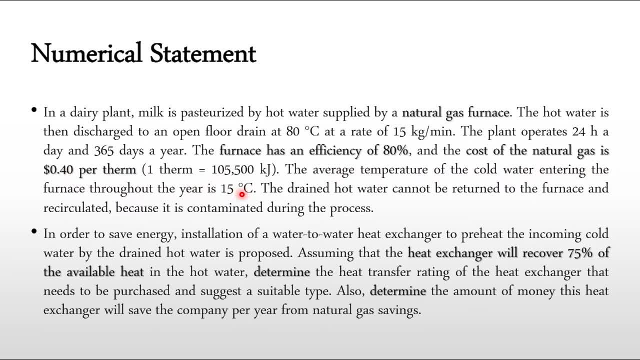 is 15 degree centigrade, so there is a furnace, the cold water is entering at 15 degree centigrade, the hot water is coming out, helping in the pasteurization of milk, and then is drained out at 80 degree centigrade and the total flow rate is 15 kg per minute of drain, the drained hot water. 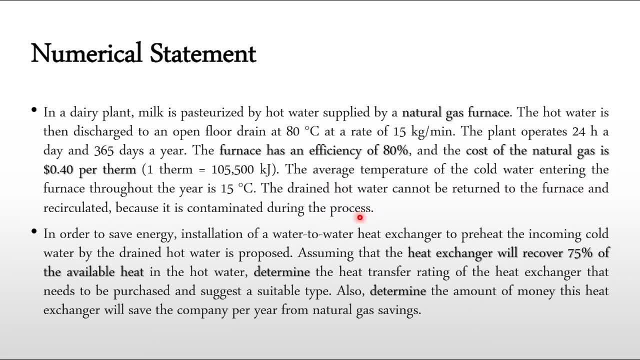 cannot be reused in the furnace because it is contaminated during the process. so the hot water is in the process, but what we can do? we can obviously preheat the cold water and that can be done by using that hot water. so what we are going to do in order to save energy, 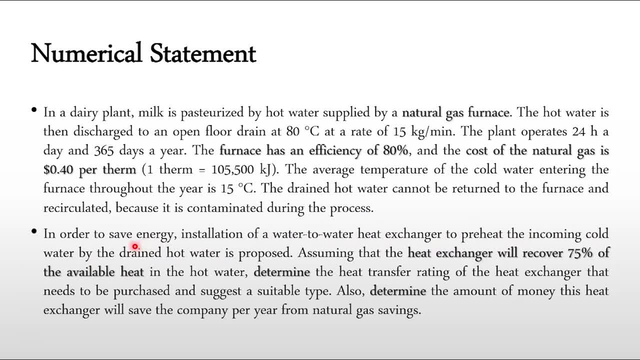 installation of water to water heat exchanger for the preheating of the incoming cold water by the drained hot water is proposed in this process, assuming that heat exchanger recovers 75 percent of the energy which is currently wasting. currently, a lot of energy is wasting. 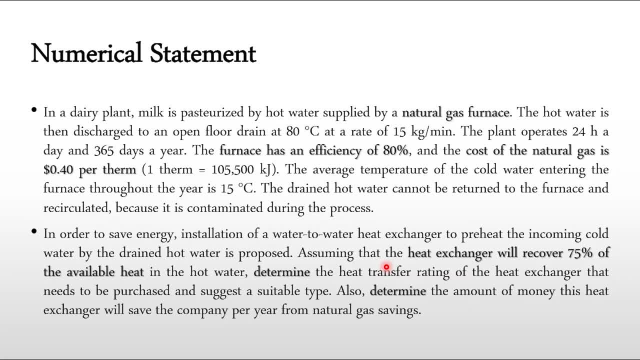 so if we are able to recover seventy five percent even energy will result in a lot of energy savings in the furnace and lot of money savings in the process. so determine the heat transfer rating of the heat exchanger that needs to be purchased and suggest a suitable type. also determine the amount of money this heat exchanger will save. 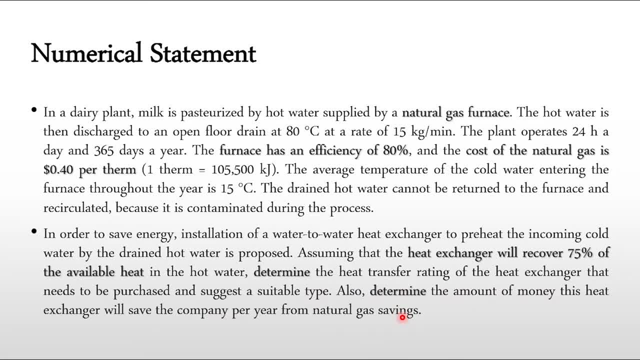 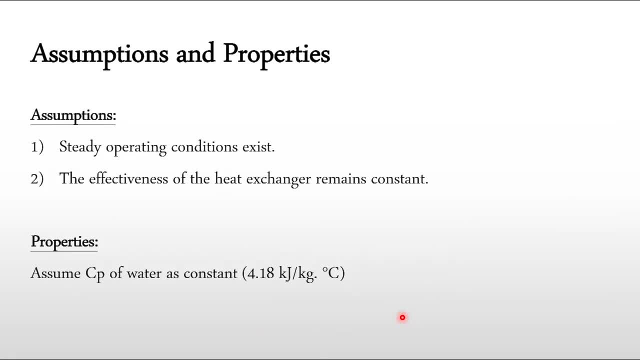 the company per year from natural gas savings. so obviously, you will save natural gas, you will save fuel, you are saving energy and, accordingly, the money will be saved. so what we need to do? there will be some assumptions and properties. the number one assumption is that the steady state conditions 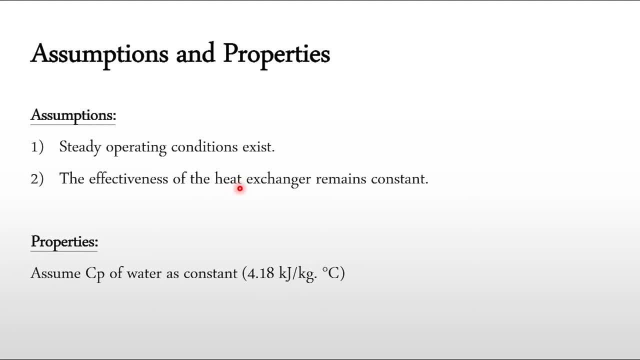 exist. number two: the effectiveness of heat exchanger remain constant, which is representing the percentage recovery: 75 percent as we have defined in the problem statement. the properties is: does assume the cpu of water as constant throughout the process as 4.18 kilojoules per. 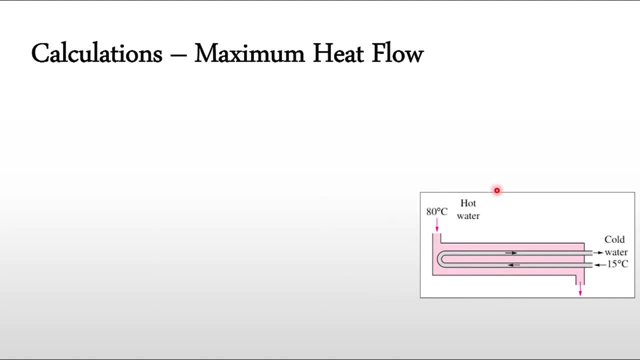 kg degree centigrade. so you can see- this is the overall representation of this heat exchanger which is proposed to be installed- that the hot water will enter this heat exchanger at 80 degree centigrade. the cold water which was earlier going directly to the furnace will fall. 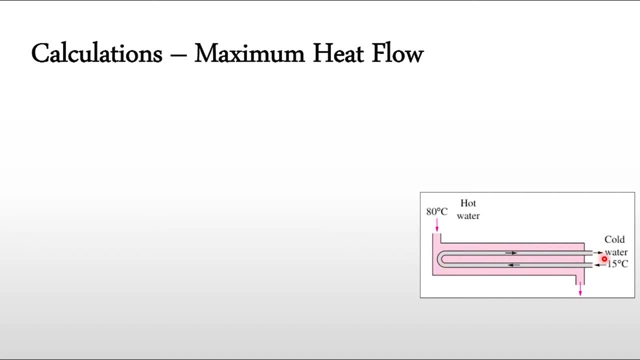 pass through this heat exchanger and the preheated cold water will then go to this furnace. so even if there is a delta of 5 or 10 degree centigrade, it will result in a lot of saving of that natural gas and, according to the energy will be saved and the energy which is currently wasting due. 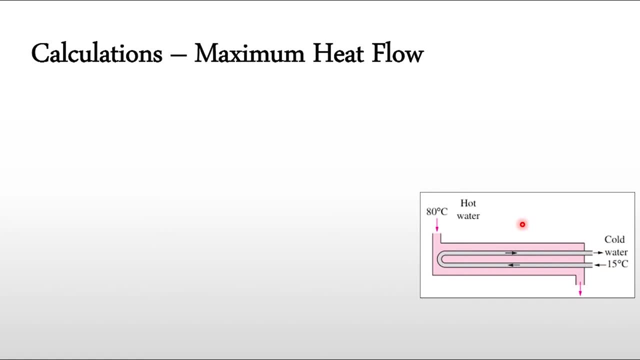 to draining of hot water will be recovered in the process as well. so first we need to calculate that, how much maximum energy that can be extracted from this hot water which is currently draining. so that is calculated as q maximum is equal to mcp, thn minus tc. as we have seen in our 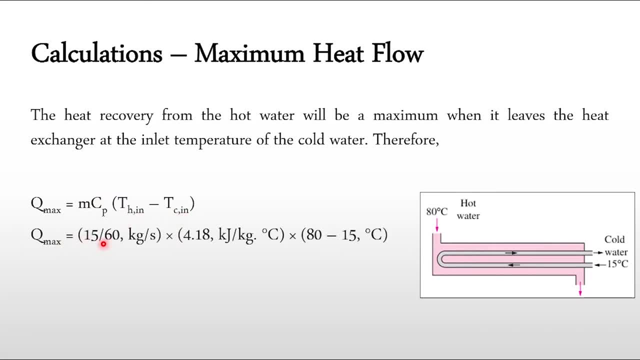 previous case. so q is equal to this one, 15 kg per minute, but that has been converted to kg per second. 4.18 kilojoule per kg degree centigrade multiplied by 80 is the inlet temperature of hot side and 15 is the temperature of cold side. so accordingly the q maximum is calculated as 67.9. 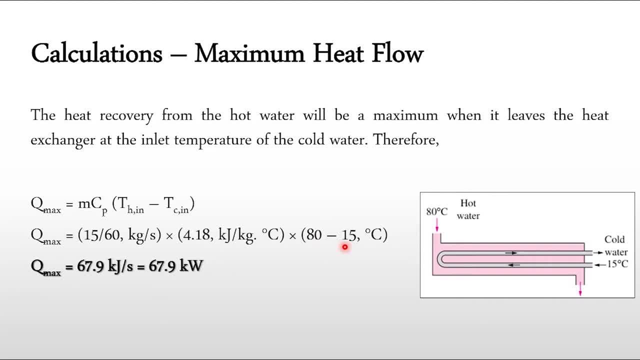 kilojoule per second, or that is equal to kilowatt. so we can say that the maximum of 67.9 kilojoule per second of heat that can be recovered from the process. but again, to recover this much heat you will be needing a high surface area of the process. so accordingly we can say that: 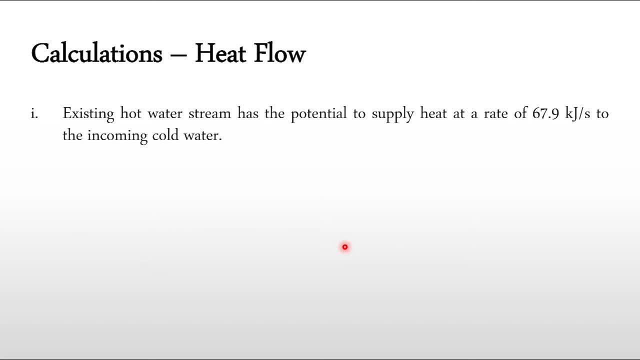 the existing hot stream water has the potential to supply heat at a rate of 67.9 second to the incoming cold water, but for this very large heat transfer surface area will be required. so what we need to do, we need to extract 75 percent of it. so what it will be becoming q is 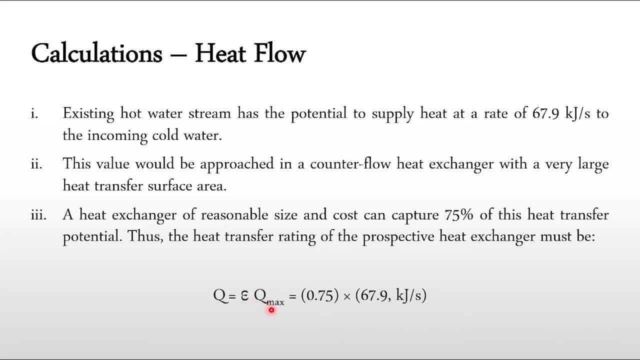 equal to effectiveness factor multiplied by q maximum, so 75 percent, multiplied by the total or the maximum amount of heat that can be extracted, so it will be 50.9 kg per second. so that's a reasonable factor that now we need to extract 50.9 kilojoule per second of the heat from the drained water and 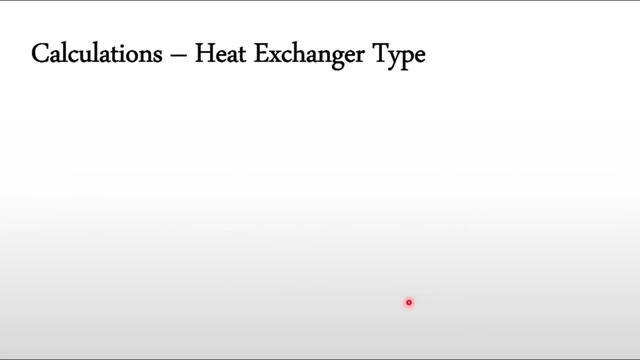 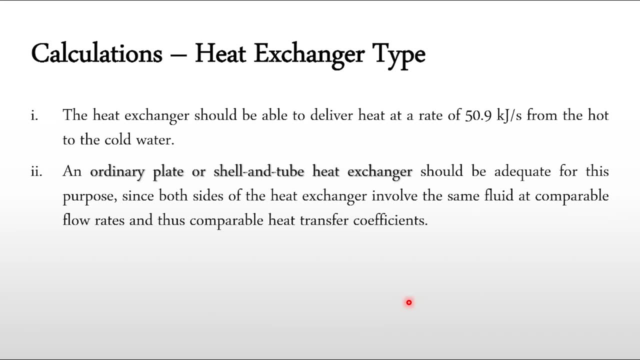 that will be supplied to the incoming water. now, what is the heat exchange type that will be able to do this? obviously, an ordinary plate or shell and tube exchanger will be good for this purpose, since both sides of the heat exchanger involve the same fluid as we have. 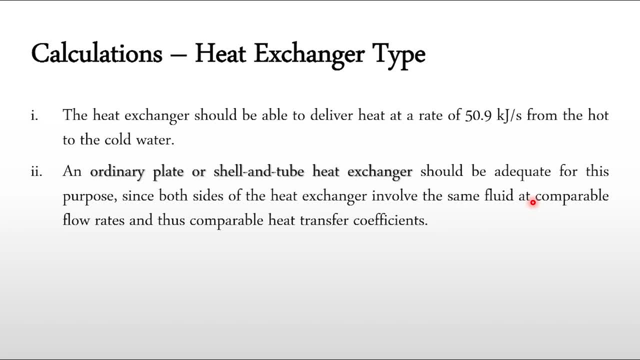 seen in platen frame. it has been said that both of the fluids should be liquid, so liquid to liquid heating and in one shell and tube can be used for this purpose as well, because there are flow rates are even same at comparable flow rates and thus comparable heat transfer coefficients. 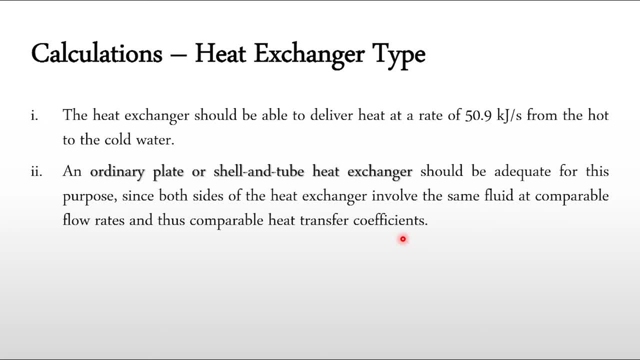 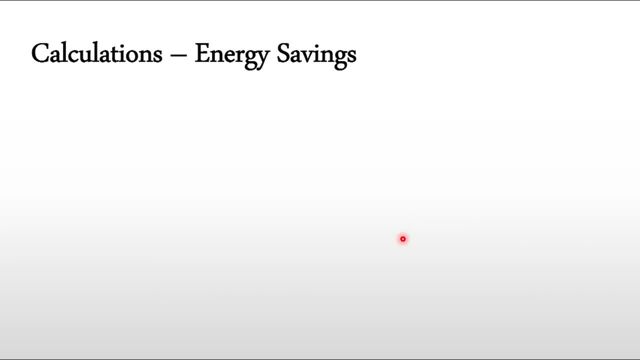 so obviously these two heat exchanger types are the suitable for this process. now we need to calculate the energy savings from the process and how that energy savings can be calculated. calculated that first we need to calculate the annual operational hours of this process and how can be calculated? obviously we have been given in the problem statement the 24 hours a day. 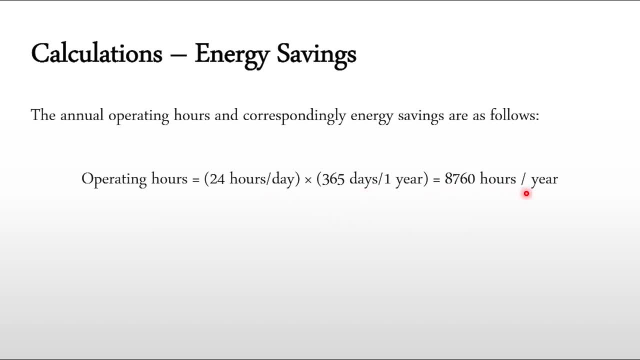 planned operation for 365 days, so accordingly the hours per years are 8760 and accordingly energy savings is equal to heat transfer rate multiplied by the operation time. heat transfer rate is 50.9 kilojoule per second. operation time is 8760 hours per year multiplying by 3600. 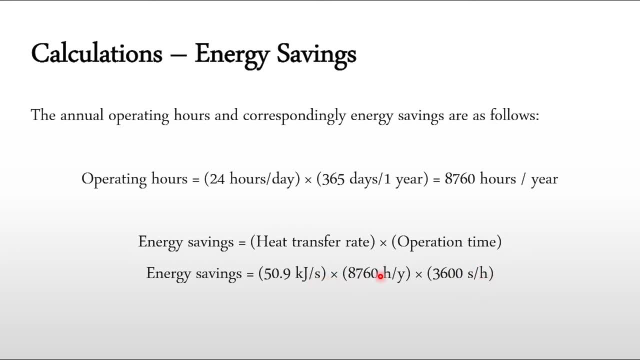 second per hour. so converting it second is cancelled out with second hour is cancelled out with this hour. so we will get answer in kilojoule per year, and that is energy savings, is equal to 1.605 multiplied by 10, raised to power, 9 kilojoule per year. so that is a total. 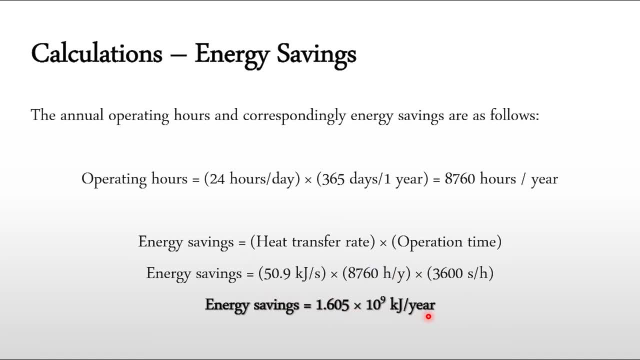 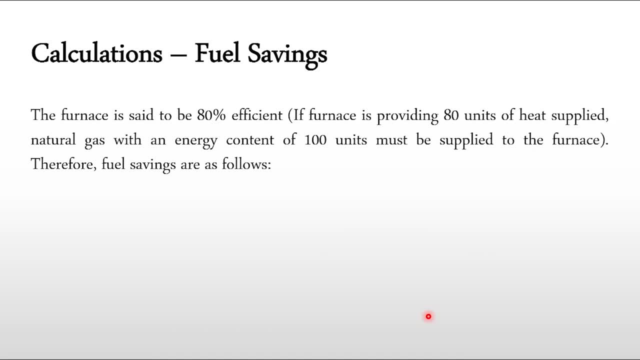 energy saving from this process. from this energy saving we can compute the fuel savings and how that can be calculated. that we have been given the furnace is 80 percent efficiency. it means that if we input the 100 units of fuel then accordingly 80 units of the heat is supplied from the furnace. so accordingly, the fuel savings, energy savings. 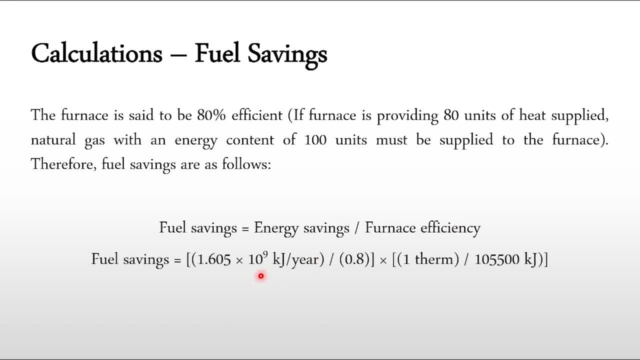 divided by the furnace efficiency. energy savings is calculated from the previous one: 1.605. multiplied by 10, raised to power 9 kilojoule per year. divided by the 0.8, which is the furnace efficiency as given in the problem statement, multiplied by one term. divided by the conversion factor, because that 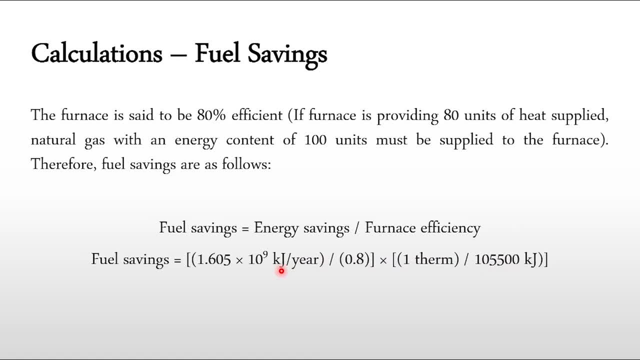 kilojoule needs to be converted into term for the fuel savings and that is the conversion factor. so now we have to calculate the money from it. so this kilojoule will be cancelled out, this kilojoule, and accordingly we get the answer in term per year, and that is equal to 19,020 terms per year. so 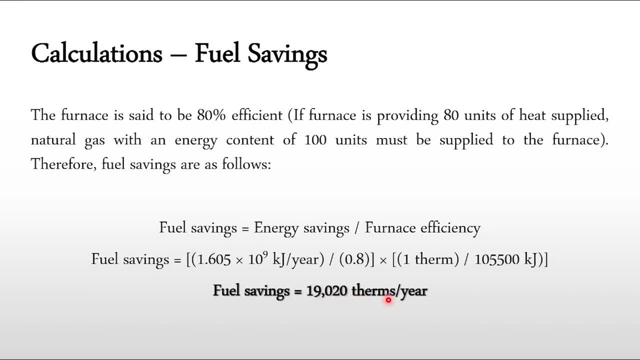 that's how the fuel savings and energy savings are calculated, and you can see that is a lot of amount that has been recovered which was earlier wasted in the process. last we need to calculate the money savings, and the price for natural gas is 0.4 dollar per.